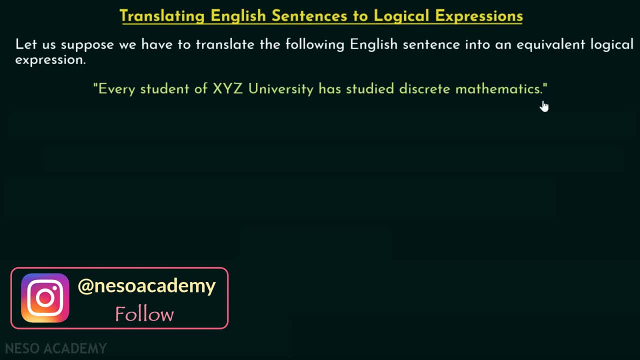 We need to translate this into an equivalent logical expression. So this statement says: every student of XYZ university has studied discrete mathematics. First, we will rewrite the statement so that we can identify the appropriate quantifiers to use. Obviously, we need to rewrite the statement so that we can identify the appropriate quantifiers. 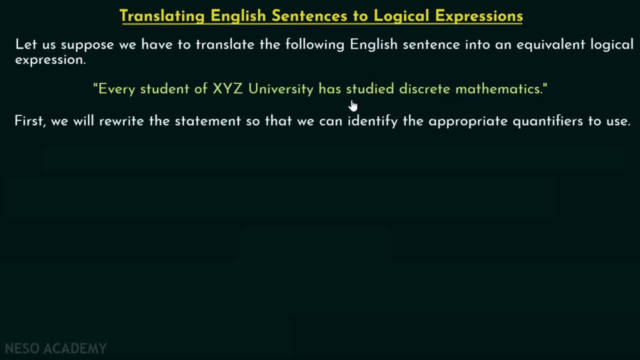 And then we can easily convert this sentence into its equivalent logical expression. So here is the rewritten statement, that is, for every student X in the XYZ university. X has studied discrete mathematics. Now let us suppose that the domain consists of all students of XYZ university. 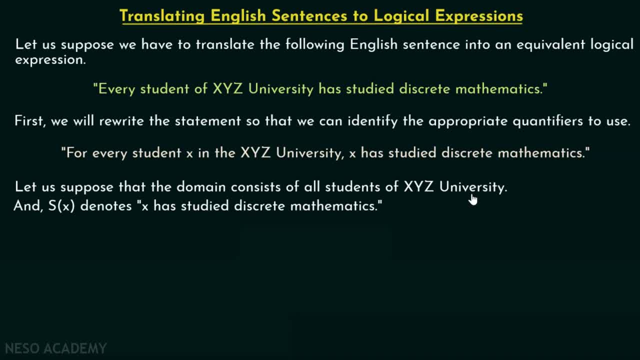 Now, this is my assumption, Obviously, I am considering this- that the domain consists of all students of XYZ university. Obviously, I am considering this: that the domain consists of all students of XYZ university And Sx denotes X has studied discrete mathematics. 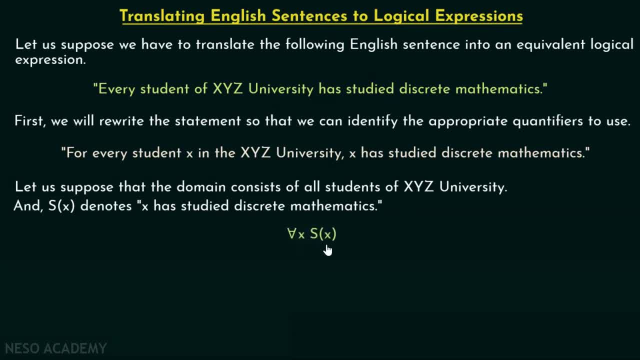 Then you can simply write this particular sentence: as for all, X, Sx, This is the equivalent logical expression of this particular sentence. Now, please note that we can also use a different domain of discourse and a set of predicates to form the equivalent logical expression of the above statement. 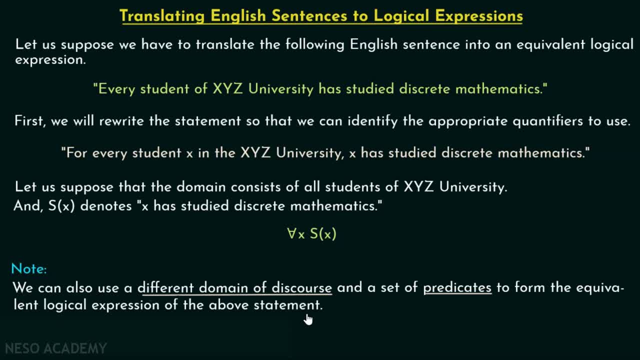 We can use a different domain of discourse and we can use a different set of predicates. There is no doubt about this right. This is my assumption, of course, that I am considering here the domain that is all students of XYZ university, But we can choose a different domain as well. 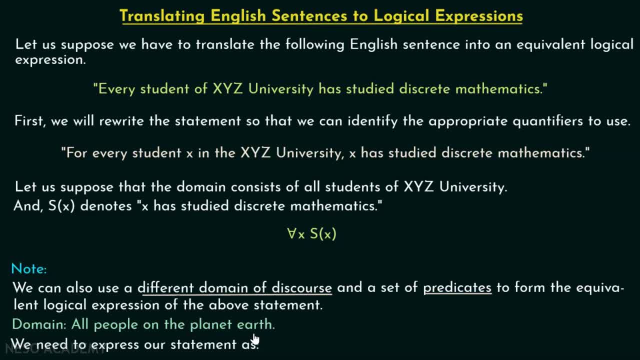 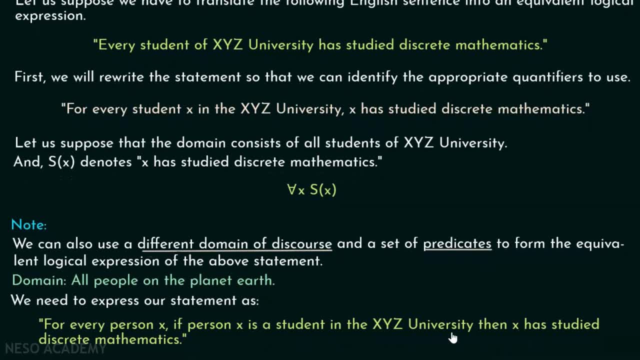 Let us say the domain is all people on the planet earth. This could be the domain, right? So we need to express our statement. as For every person X, If person X is a student in the XYZ university, then X has studied discrete mathematics. 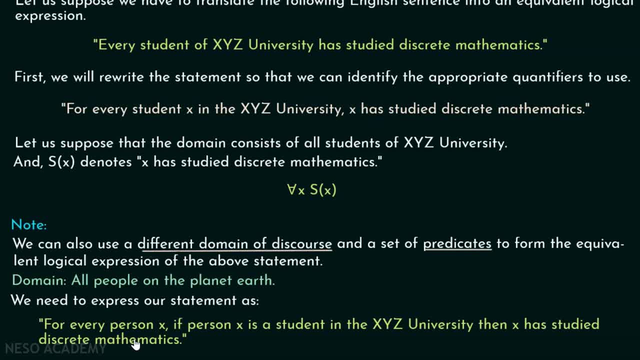 So here I am considering the domain as all people on the planet earth. That is why I have to make a selection For every person. X x is a student in the xyz university. This is very important. We need to make the selection. 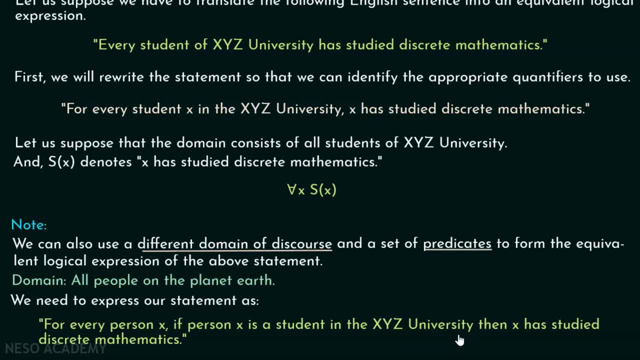 right, Because we can't say that every person x has studied discrete mathematics. We have to select students of the xyz university from all people on the planet earth, right? That is why the selection is required and this means implication is required. So if person x is a student in the 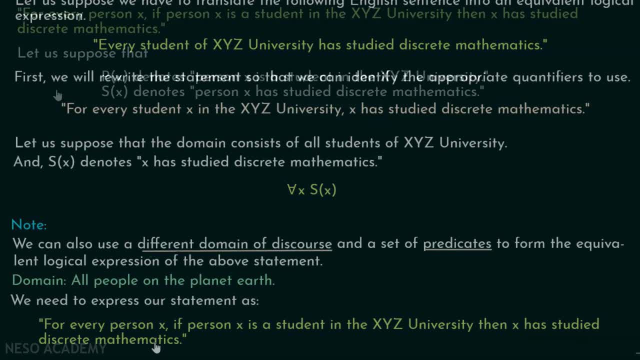 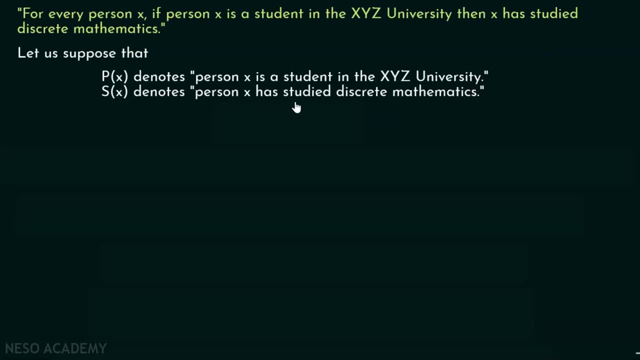 xyz university, then x has studied discrete mathematics. Now let us suppose that Px denotes person x is a student in the xyz university and Sx denotes person x has studied discrete mathematics. Then we can rewrite this sentence as for all x, Px implies Sx. Here the sentence is: 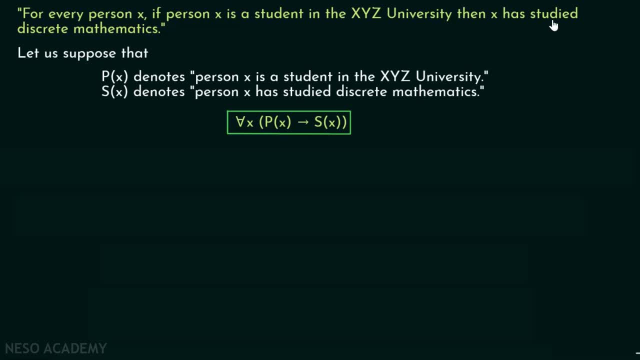 for every person x. if person x is a student in the xyz university, then x has studied discrete mathematics. This means implication came into picture, right? So here for all x quantifier will be used, and of course here we will use this predicate Px, and Px implies Sx, If x is a student. 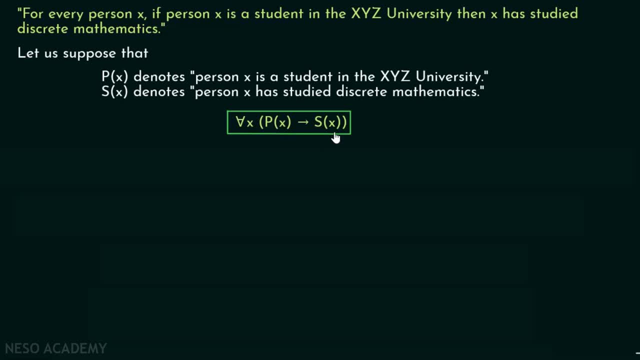 in the xyz university, then x has studied discrete mathematics. So here for all, x quantifier will be used, and of course here we will use this predicate Px, and Px implies Sx. If x is a student in the xyz university, then x has studied discrete mathematics. As simple as that. Now please note. 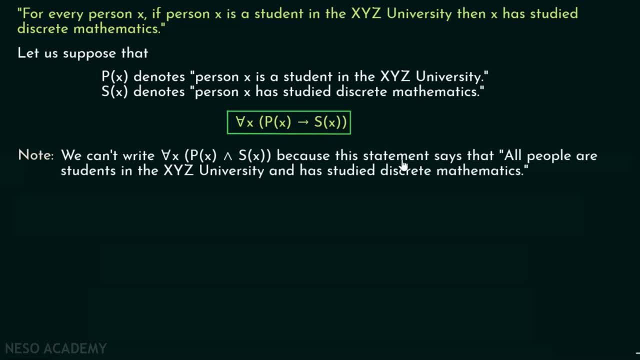 that we can't write for all x, Px and Sx, because this statement says that all people are students in the xyz university and has studied discrete mathematics. That is, all people on the planet earth are actually the students of xyz university and has studied discrete mathematics. It does not. 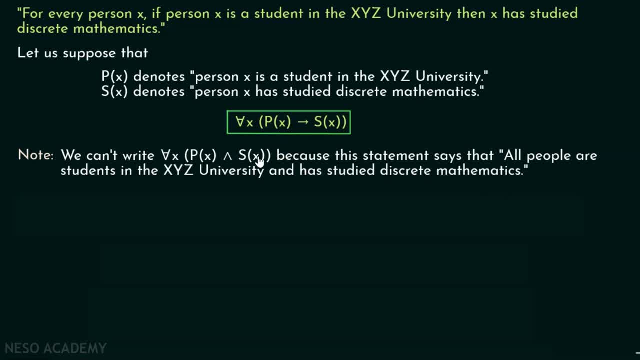 make any sense right. That is why we can't use for all x, Px and Sx. We can also use a two variable predicate, like this: Sx comma y, which represents the number of students in the xyz university and represents the statement person x has studied subject y. Like this, for all x, Px. 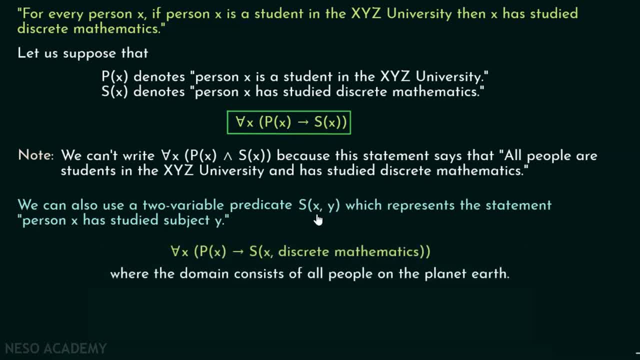 implies Sx comma, discrete mathematics. This is a two variable predicate which represents the statement person x has studied subject y. If x is a student in the xyz university, then x has studied discrete mathematics. Now, here the domain consists of all people on the planet earth, While 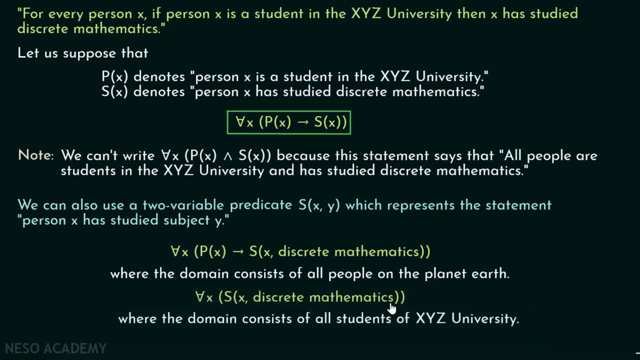 we can also write for all x, Sx, comma discrete mathematics, if the domain consists of all students of xyz university. That's a simple thing. Now let's see how we can write for all x, Px and Sx. So it is a matter of choice whether you will take a one variable predicate or two variable. 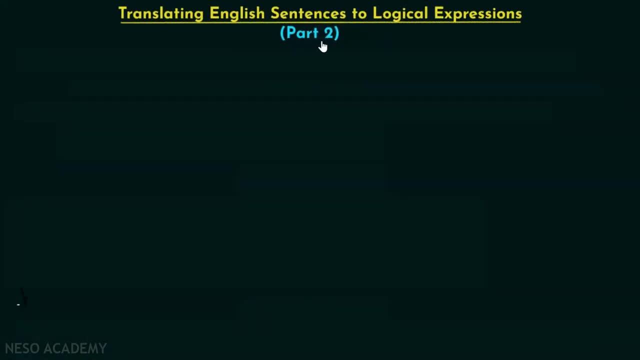 predicate. It's your choice. okay, Let us consider part two of translating English sentences to logical expressions. Let us suppose that we want to translate the following into logical expressions: So this is the sentence and we need to translate this into an equivalent logical expression. 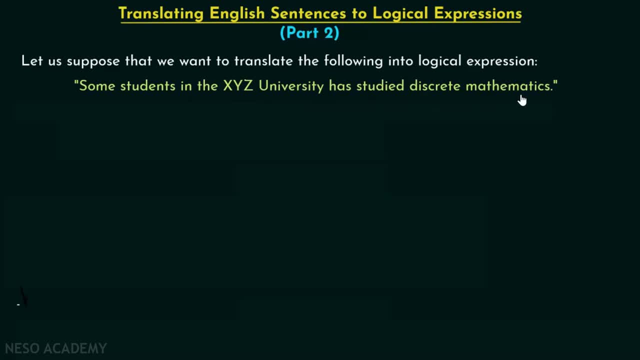 Some students in the xyz university has studied discrete mathematics. Now let us consider the domain of all students of xyz university, and I am considering the predicate Px, as x has studied discrete mathematics. So we can translate this English sentence into its equivalent logical expression, which looks like this: There exists x- Px, So this is an equivalent logical expression. 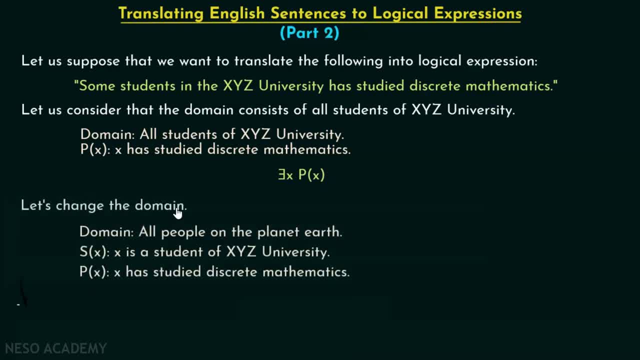 of this particular English sentence. Let's change the domain. Domain consists of all people on the planet earth. You can change the domain anytime, that doesn't matter. okay, But if the domain is changed, then the predicates may change, okay. So let's change the domain of all students of xyz university. 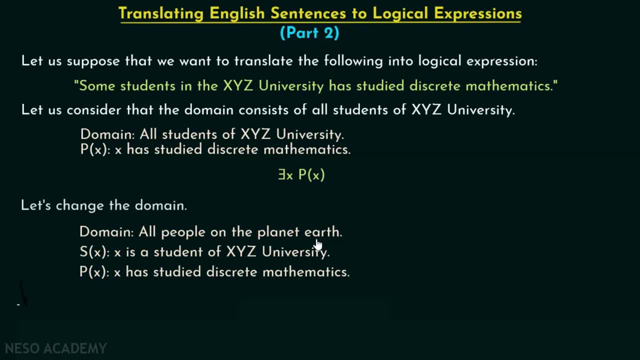 So you need to take care about the predicates and the logical expression so formed must be well formed. Let us suppose Sx denotes x is a student of xyz university and Px denotes x has studied discrete mathematics. Then you can rewrite this statement as there exists x, Sx and Px Now here. 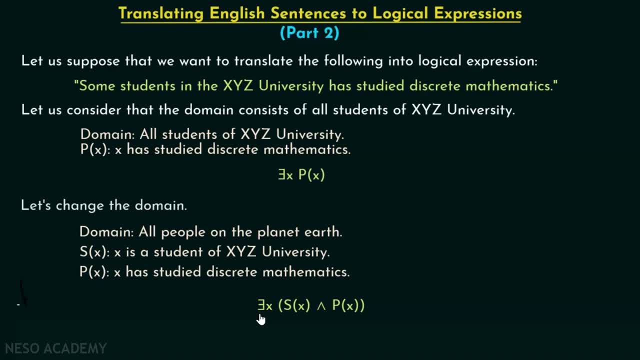 and will come into picture because we are considering this particular quantifier. there exists. It denotes there is some person x having the properties that x is a student of xyz university and x has studied discrete mathematics. So this is very important. We are considering some person x who is the student of xyz university. 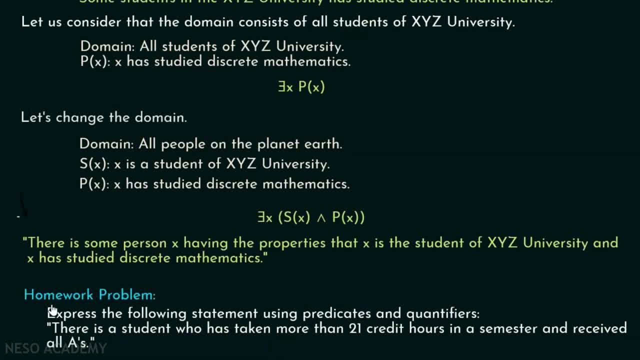 and who has also studied discrete mathematics. Now let us consider one homework problem. Express the following statement using predicates and quantifiers: There is a student who has taken more than 21 credit hours in a semester and received all A's. You need to express this. 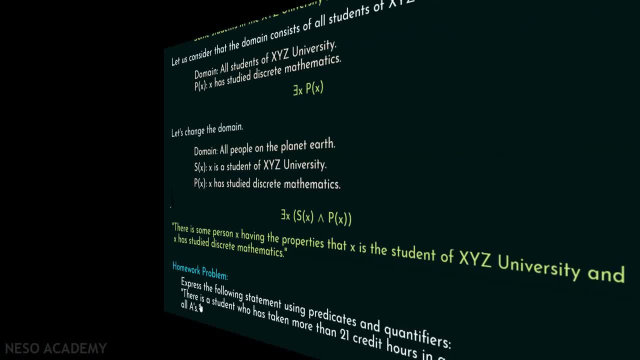 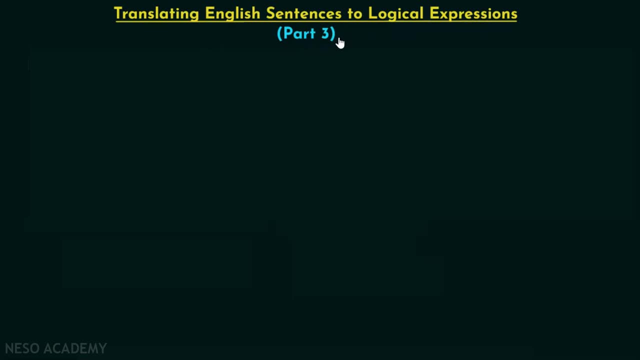 statement using predicates and quantifiers. okay, Let's discuss part three of translating English sentences to logical expression. Here we will discuss one problem statement And we will try to find out the solution for that problem. Consider these statements: The first two: 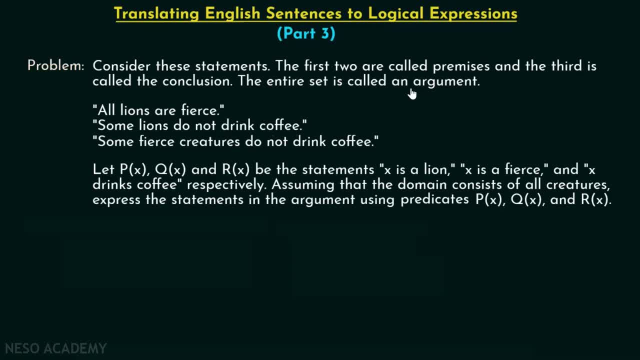 are called premises and the third is called the conclusion. The entire set is called an argument. So this is the entire set which is called an argument. The third one is the conclusion, and these two are the premises. All lines are fierce. Some lines do not drink coffee. Some fierce. 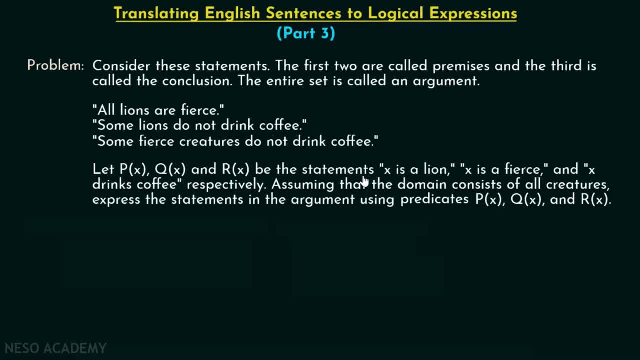 creatures do not drink coffee, Let Px, Qx and Rx be the statements x is a lion, x is a fierce and x drinks coffee respectively. okay, Assuming that the domain consists of all creatures, express the statements in the argument using predicates Px, Qx and Rx. So 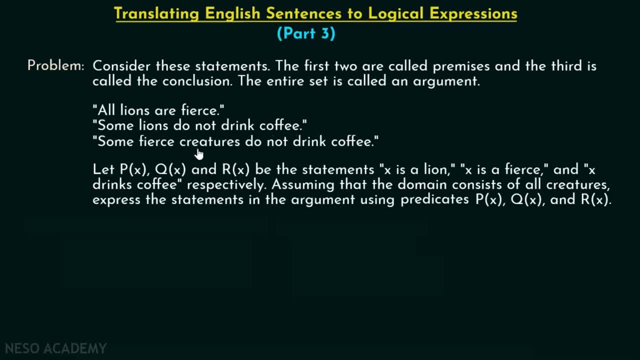 basically we need to translate these English sentences into their equivalent logical expressions: So here the domain consists of all creatures, right? It is given in the question that, assuming that the domain consists of all creatures, So here the domain is all creatures. Px denotes x is. 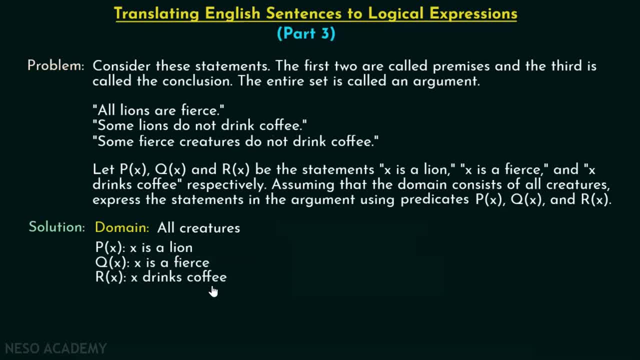 a lion, Qx denotes x is a fierce and Rx denotes x drinks coffee. We can write the first sentence for all x, Px implies Qx. Here, of course, for all quantifier will come because we are talking about all lions, right, And because x denotes all creatures, so we have to select lions from. 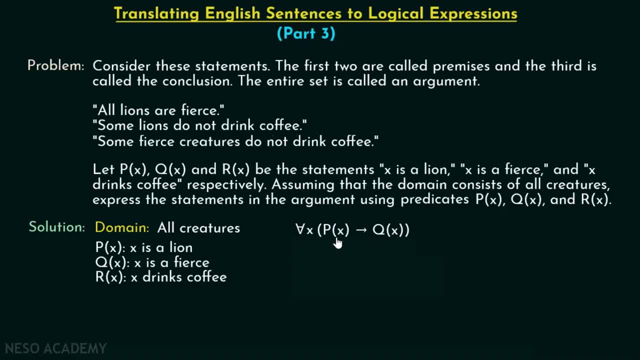 all the creatures. For this we need this predicate Px, because Px denotes x is a lion. Now here. this statement means: if x is a lion, then x is a fierce. This means all lions are fierce. Now let's try to. 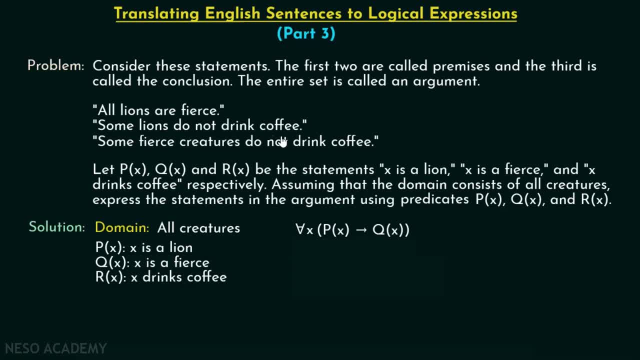 convert this sentence. Some lions do not drink coffee, So here we will use their exist quantifier. So Rx denotes x drinks coffee. So not of Rx denotes x do not drink coffee. because we are considering that there exist quantifier and will come into picture. Now let's try to convert this. 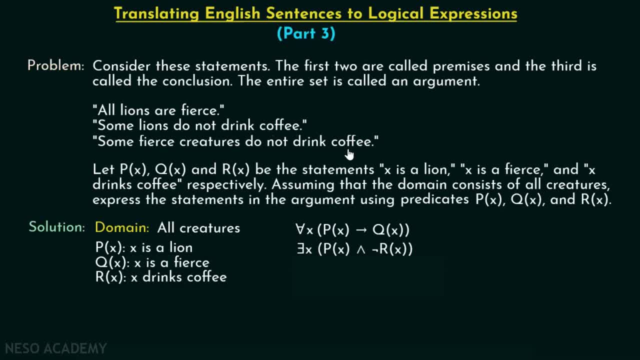 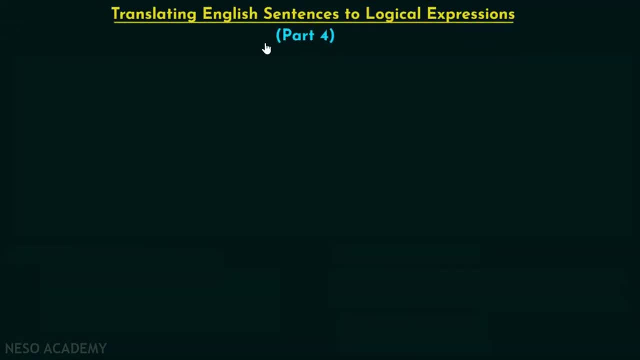 sentence: Some fierce creatures do not drink coffee. So the logical expression corresponding to this particular sentence is: there exist x, Qx and not of Rx. Let's discuss part 4 of translating English sentences to logical expressions. Here we will consider one problem. Consider these: 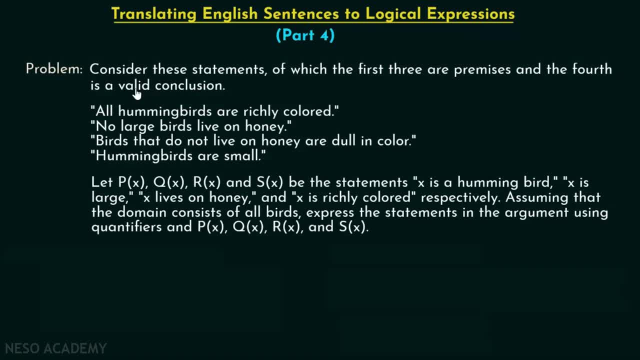 statements, of which the first three are premises and the fourth is a valid conclusion. So these are the three premises- the first three and the last one is the conclusion. All hummingbirds are richly colored. No large birds live on honey. Birds that do not live on honey are dull in color. 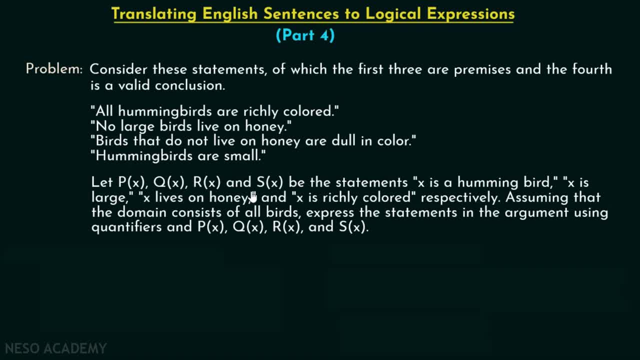 Hummingbirds are small, Let Px, Qx, Rx and Sx be the statements x is a hummingbird, x is large, x lives on honey and x is richly colored, respectively, Assuming that the domain consists of all birds. express the statements in the argument using quantifiers and, of course, these: 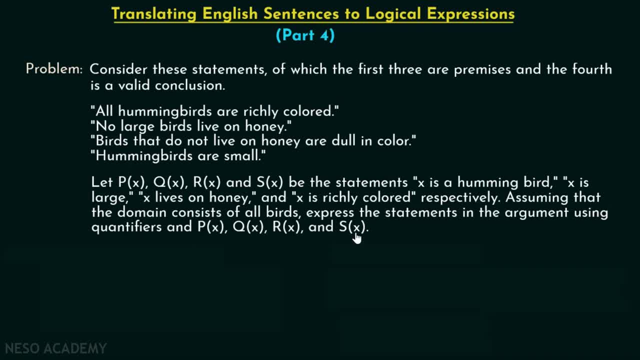 predicates Px, Qx, Rx and Sx. So here comes the solution. The domain consists of all birds right, and these are the predicates: Px, Qx, Rx and Sx. Px denotes x is a hummingbird, Qx denotes x is large. 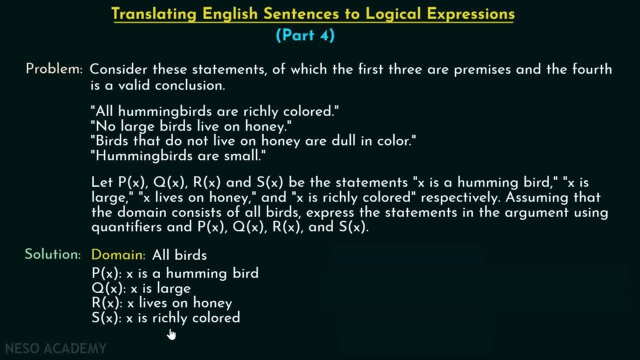 Rx denotes x lives on honey and Sx denotes x is richly colored. So the first statement can easily be converted in this form. that is for all: x. Px implies Sx. This is simple, because here Px denotes it and Sx denotes x is richly colored. Now here, because we are talking about all hummingbirds. 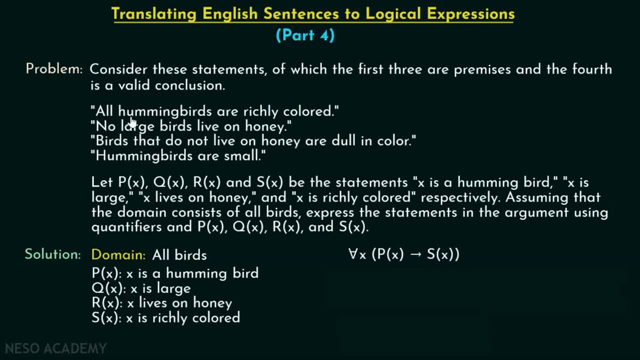 that's why for all quantifier will come into picture. and we are talking about all hummingbirds are richly colored. If x is a hummingbird, then x is richly colored. Now let's consider the second statement. No large birds live on honey Here. this can be converted to for all x. Qx implies not of 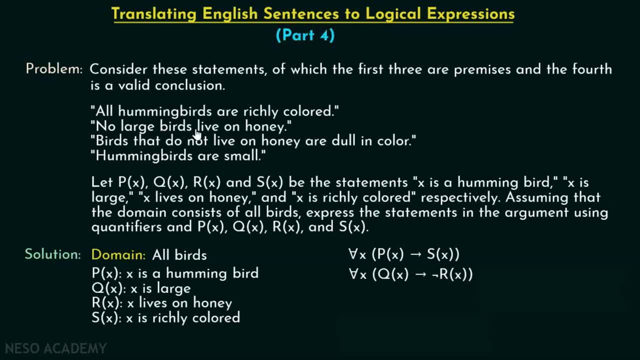 Rx, Isn't that so? Because you are talking about large birds, so obviously we have to take Qx, not live on honey. Now, in order to understand this logical expression in a better way, I will convert this logical expression in the form which is easily understandable. Okay, so here. first we 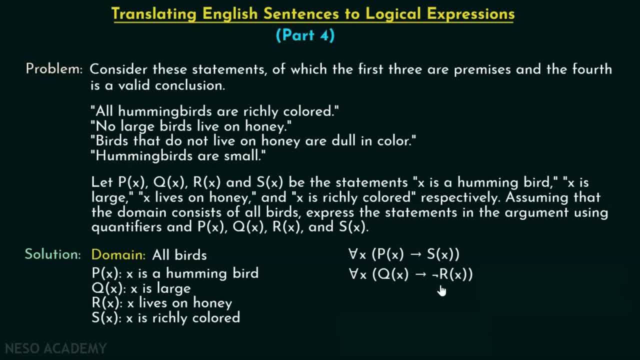 will convert this implication. that is, we know that P implies Q means not of P or Q. So let's write in this form: that is not of P or Q, and then after that I will move this negation outside, which means this or becomes, and and obviously these negations will get cancelled. So this negation comes. 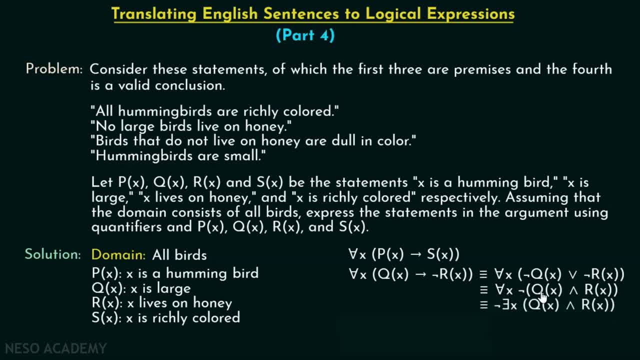 next step. So this becomes: there exist x. Now please read this particular logical expression that is not of there exist x, Qx and Rx. What does it mean? It means that it is not the case that there exists some bird which is large in size and which lives on honey. So this is the sentence. so 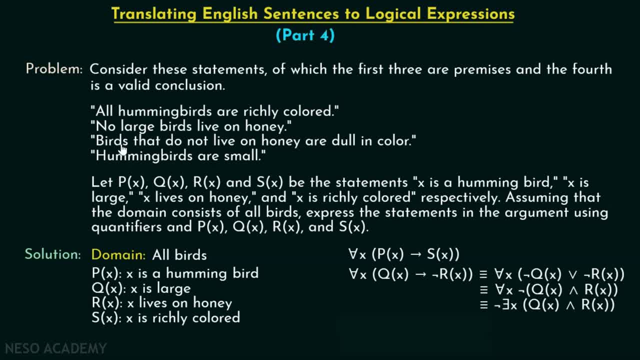 far and now it makes sense. right Now. let's consider the third statement, that is, birds that do not live on honey are dull in color. Okay, so we were talking about birds that do not live on honey. Of course, we have to take this predicate. 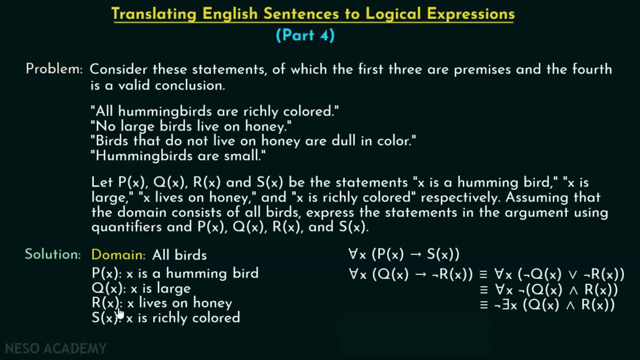 that is Rx and dull in color, because we do not have anything like dull in color. So we'll take this Sx which says x is richly colored, and we'll take the negation of this Sx right. So this is. 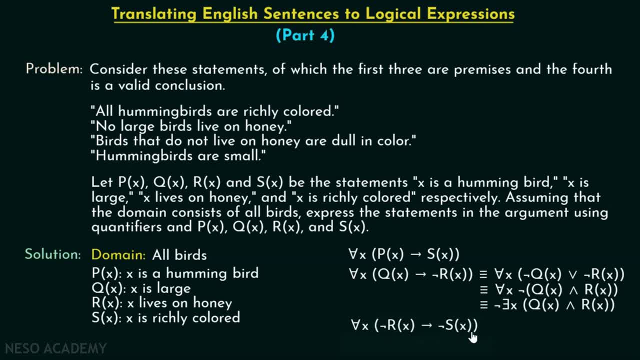 how the statement looks like for all. x not of Rx implies not of Sx, right? Not of Rx means that birds that do not live on honey, right? So here, if x does not live on honey, then x is not richly colored, or I can say x is dull in color. Now, after this, we have hummingbirds are small, We're. 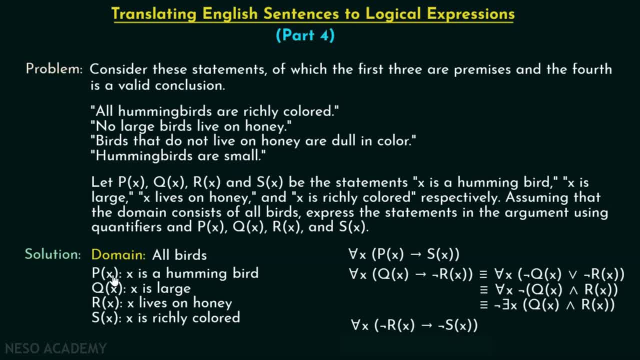 talking about all the hummingbirds. okay, So here we will take the Px predicate, of course, and of course we have to take this Qx predicate as well. So this sentence can be converted. as for all x, Px implies not of Qx, right? So